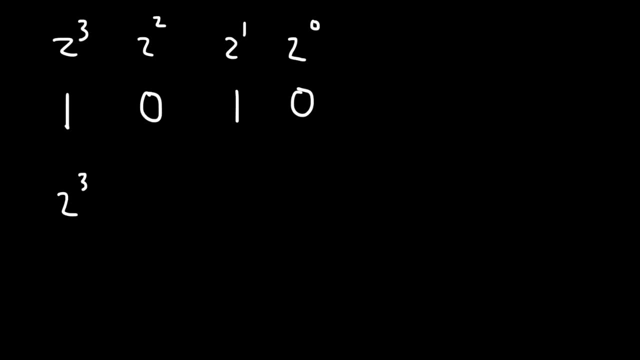 And then 2 to the 3rd power, And then, if we multiply 2 squared by 0, that's going to give us 0. And we're going to add these values And then it's going to be 1 times 2 to the 1st power, which is just 2 to the 1st power. 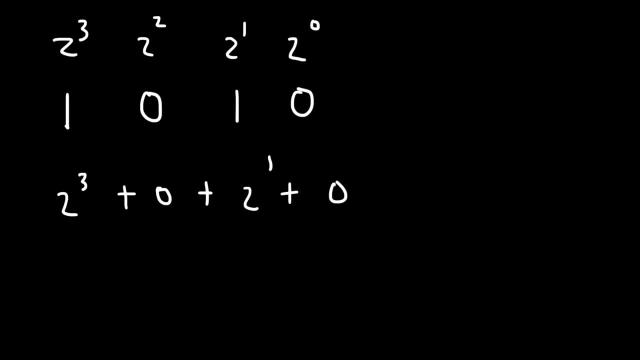 And then 0 times 2 to the 0 is 0. So everywhere you see a 0, you could ignore it, So we only need to focus on the numbers that contain a 1.. Now let's add up these numbers. 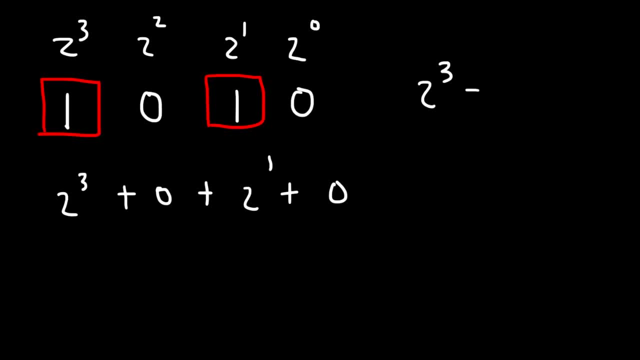 So what is 2 to the 3rd power? 2 to the 3rd power is 2 times 2 times 2,, which is 8.. 2 to the 1st power is simply 2.. So we're going to get 8 plus 2.. 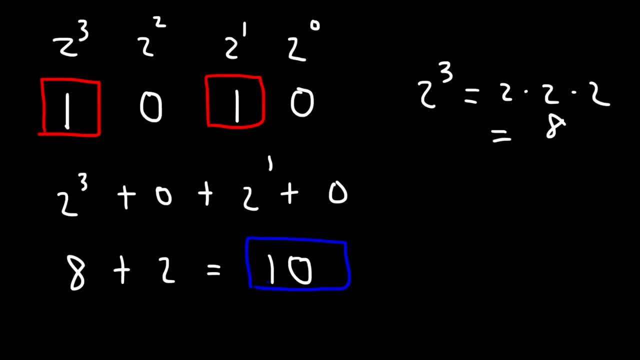 And so the answer is 10.. So the binary number 1010 has a value of 10.. Now let's try another example: 10010.. So if you want to try it, feel free to pause the video. Go ahead and write this number down and convert the binary number into a decimal number. 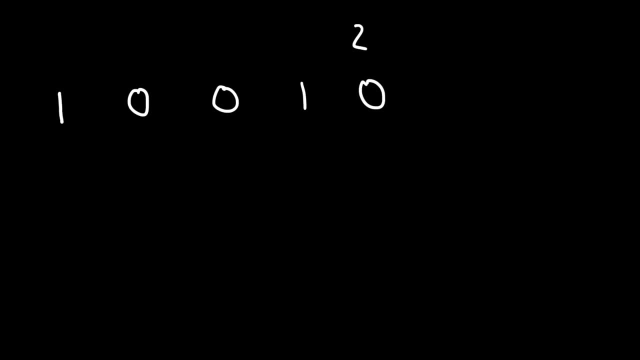 So let's start from the right side. This is going to be 2 to the 0 power. The next number is 2 to the 1st power. It's 0 times 2 to the 0,, by the way. 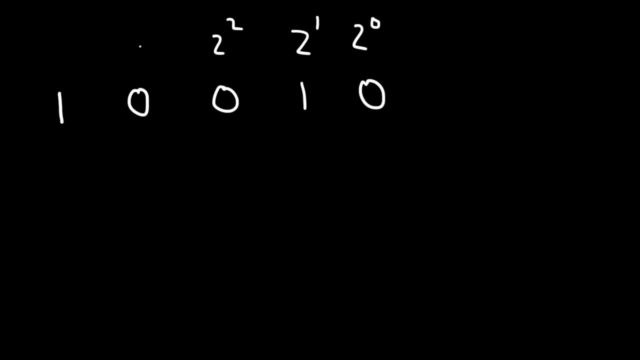 And then the next number is going to be 0 times 2 squared, And then 0 times 2 to the 3rd, And then 1 times 2 to the 4th. Now we don't need to worry about the 0s. 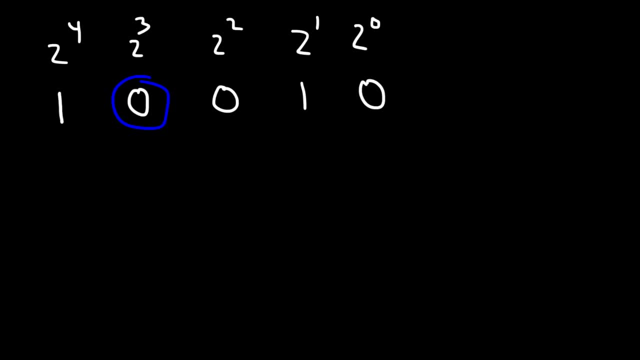 So let's ignore those numbers. Focus on the numbers that have a 1. Because those numbers will contribute to the final answer. So this is going to be 1 times 2 to the 4th power, which is simply 2 to the 4th power. 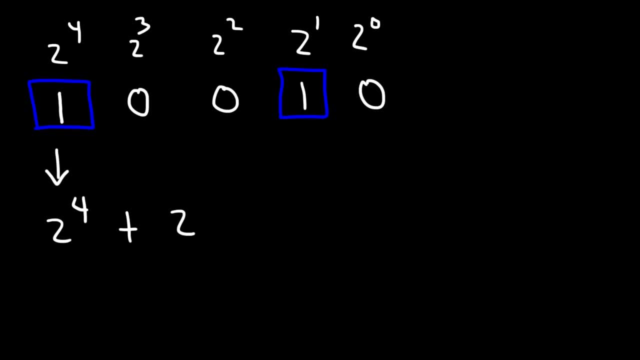 And then this is 1 times 2 to the 1st power, which is just 2 to the 1st power. So what is 2 to the 4th power? So 2 to the 4th power is 1 times 2 to the 1st power. 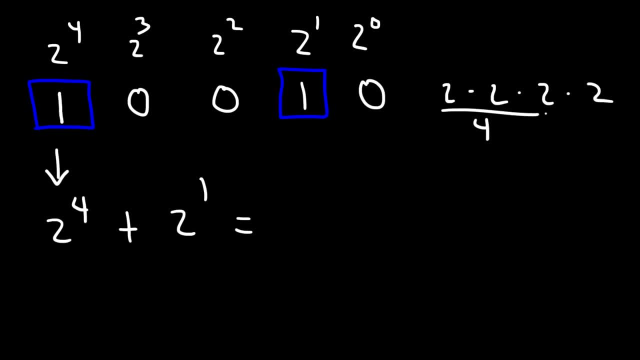 So 2 to the 4th power is 1 times 2 to the 1st power. So 2 times 2 times 2 times 2.. 2 times 2 is 4.. And 4 times 4 is 16.. 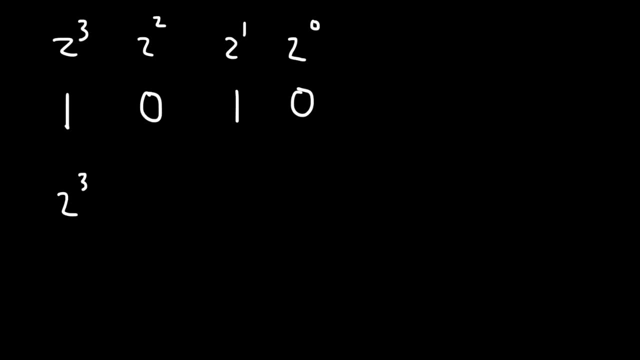 And then 2 to the 3rd power, And then, if we multiply 2 squared by 0, that's going to give us 0. And we're going to add these values And then it's going to be 1 times 2 to the 1st power, which is just 2 to the 1st power. 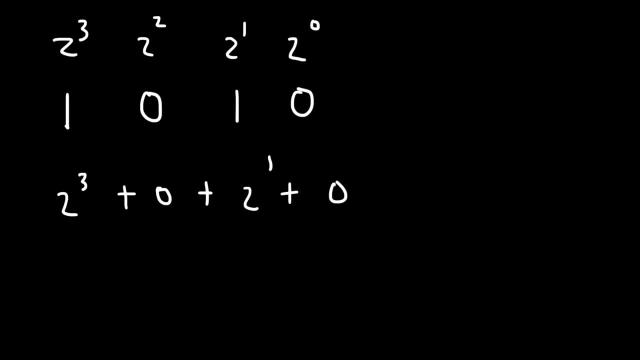 And then 0 times 2 to the 0 is 0. So everywhere you see a 0, you could ignore it, So we only need to focus on the numbers that contain a 1.. Now let's add up these numbers. 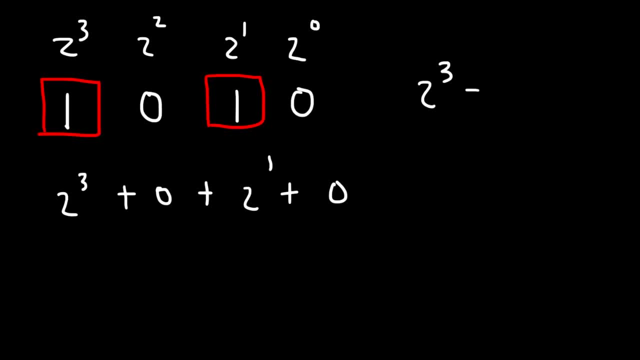 So what is 2 to the 3rd power? 2 to the 3rd power is 2 times 2 times 2,, which is 8.. 2 to the 1st power is simply 2.. So we're going to get 8 plus 2.. 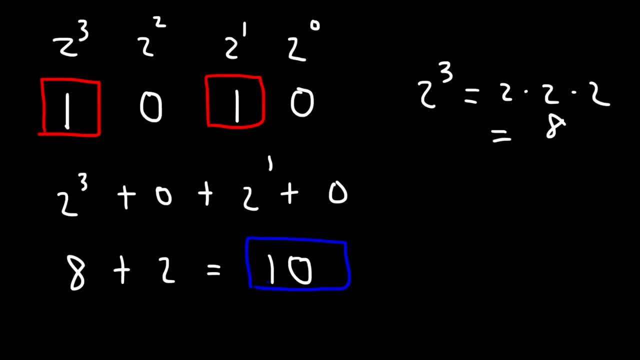 And so the answer is 10.. So the binary number 1010 has a value of 10.. Now let's try another example: 10010.. So if you want to try it, feel free to pause the video. Go ahead and write this number down and convert the binary number into a decimal number. 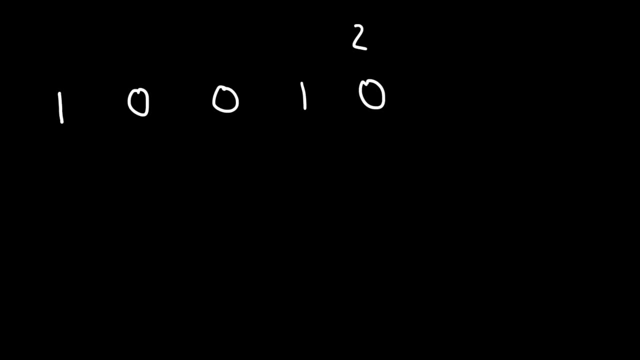 So let's start from the right side. This is going to be 2 to the 0 power. The next number is 2 to the 1st power. It's 0 times 2 to the 0,, by the way. 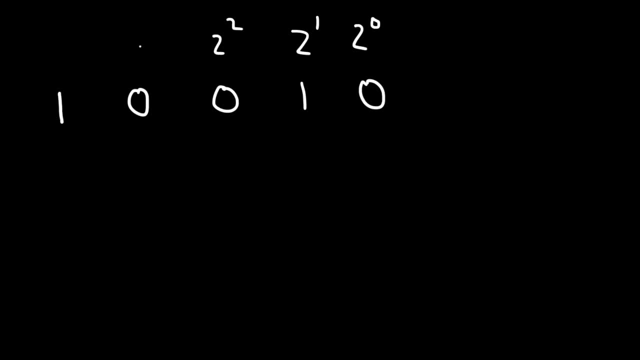 And then the next number is going to be 0 times 2 squared, And then 0 times 2 to the 3rd, And then 1 times 2 to the 4th. Now we don't need to worry about the zeros. 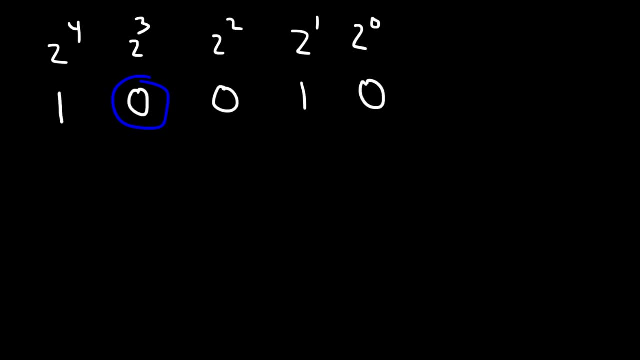 So let's ignore those numbers. Focus on the numbers that have a 1. Because those numbers will contribute to the final answer. So this is going to be 1 times 2 to the 4th power, which is simply 2 to the 4th power. 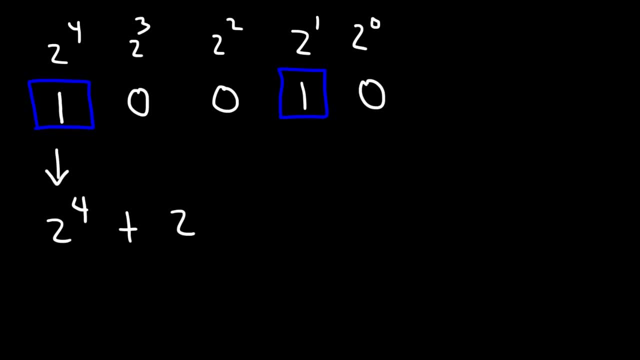 And then this is 1 times 2 to the 1st power, which is just 2 to the 1st power. So what is 2 to the 4th power? So 2 times 2 to the 1st power is 1.. 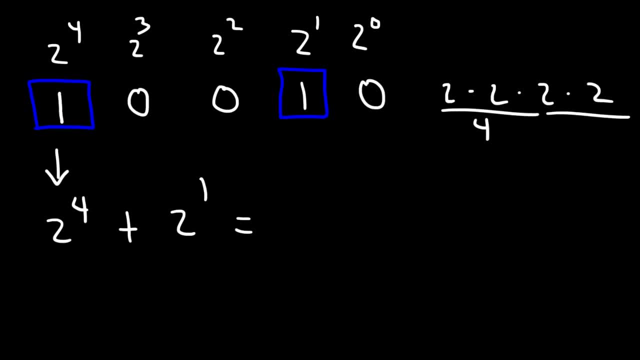 2 times 2 times 2 times 2.. 2 times 2 is 4. And 4 times 4 is 16.. So 2 to the 4th power is 16. Plus 2. And so this will give us 18.. 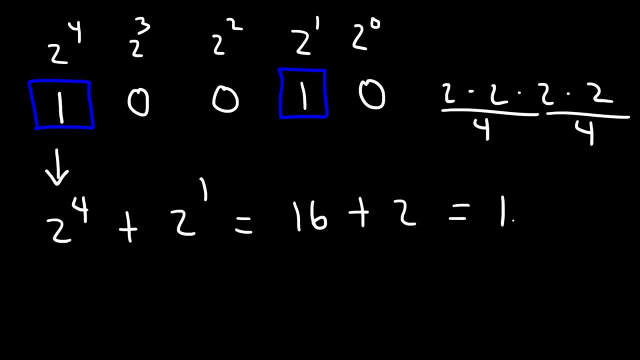 So 2 to the 4th power is 16. Plus 2. And so this will give us 18. And so it's not very difficult to convert a binary number into a decimal number. As long as you follow the process, you're going to get this right. 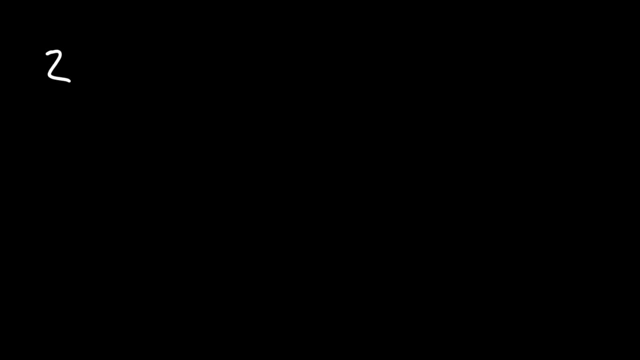 Now here's some information that you may want to know. 2 to the 0 power Is 1.. In fact, anything raised to the 0 power is 1.. 2 to the 1st power is 2.. 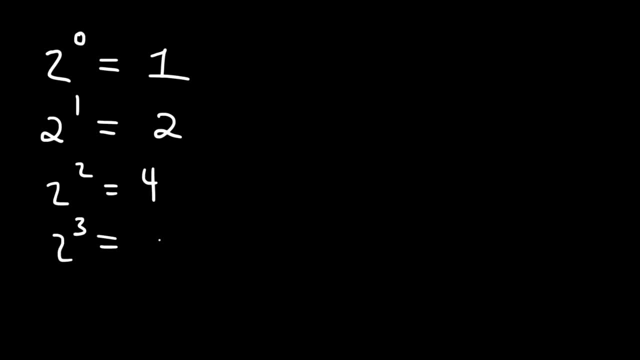 2 squared is 4.. 2 to the 3rd is 8.. 2 to the 4th is 16.. And then 2 to the 5th power, that's 32.. 2 to the 6th is 64.. 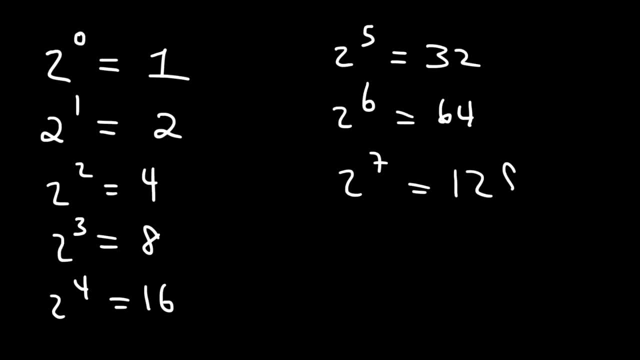 2 to the 7th is- uh, that's 128.. And then 2 to the 8th is 128 times 2, or 256.. And so if you know these values, you can quickly perform the operations that's necessary when converting a binary number into a decimal number. 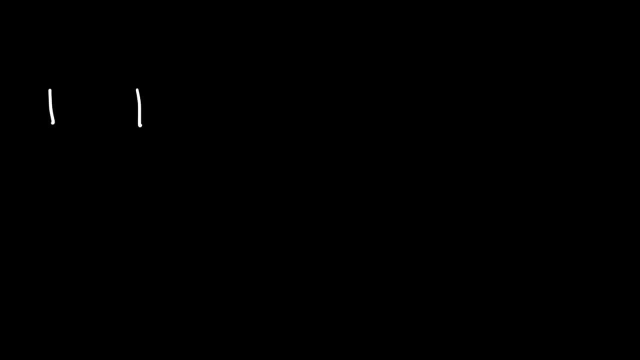 So let's try another example: 1, 1, 0, 1, 1.. So go ahead and convert this number into a decimal number. So this is going to be 2 to the 0 times 1.. And then 2 to the 1st power times 1.. 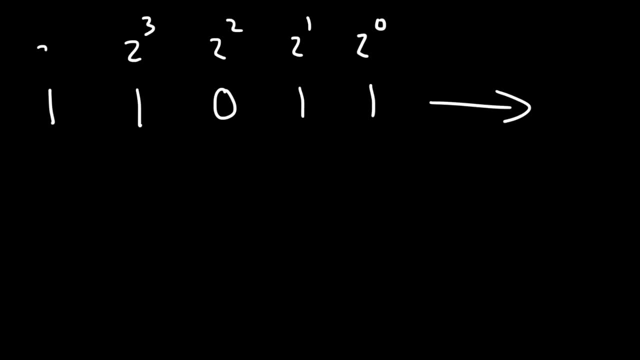 2 squared times 0.. 2 squared times 1.. 2 squared times 0.. 2 to the 3rd times 1.. And then 2 to the 4th times 1.. And, just like before, we are going to ignore the 0 values and focus on the numbers that have a binary value of 1.. 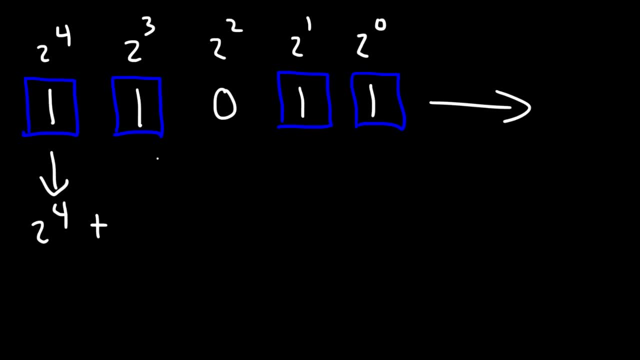 So this is going to be 2 to the 4th And then plus 2 to the 3rd power, And then plus 2 to the 1st And then plus 2 to the 0 power. So based on that table, or rather, 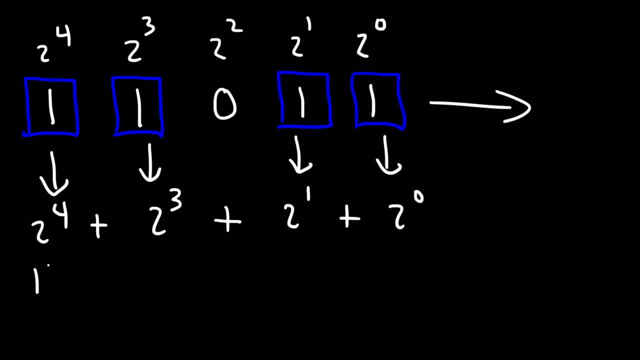 the information on the last page, we said that 2 to the 4th power is 16.. 2 to the 3rd is 8.. 2 to the 1st is 2. And 2 to the 0 is 1.. 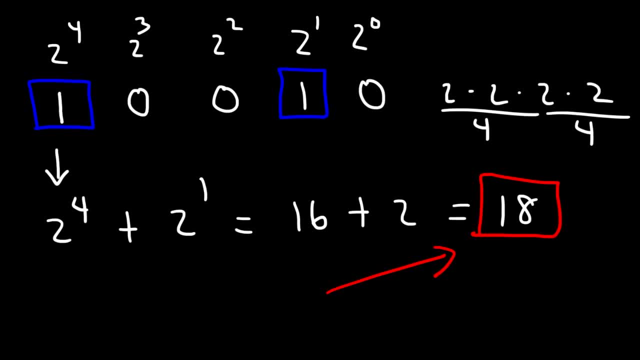 And so it's not very difficult to convert a binary number into a decimal number. As long as you follow the process, you're going to get this right. Now here's some information that you may want to know. 2 to the 0 power. 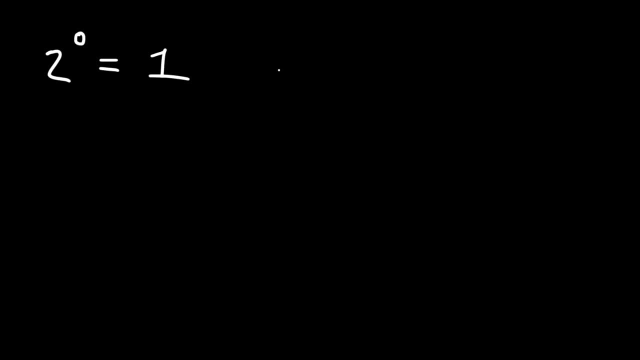 Is 1.. In fact, anything raised to the 0 power is 1.. 2 to the 1st power is 2.. 2 squared is 4.. 2 to the 3rd is 8.. 2 to the 4th is 16.. 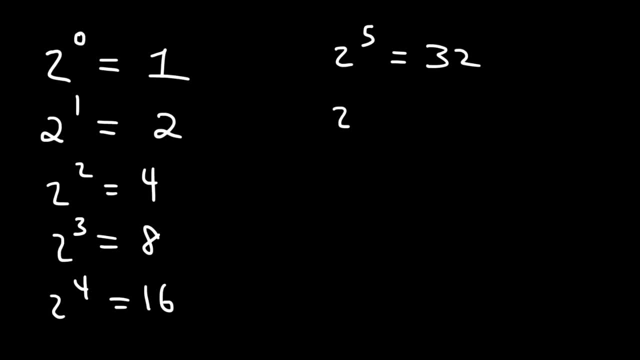 And then 2 to the 5th, power, that's 32.. 2 to the 6th is 64.. 2 to the 7th is that's 128.. And then 2 to the 8th is 128 times 2, or 256. 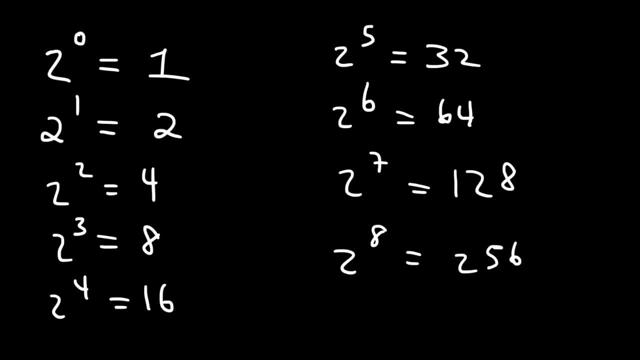 256.. And so if you know these values, you can quickly perform the operations that's necessary when converting a binary number into a decimal number. So let's try another example: 1, 1, 0, 1, 1.. 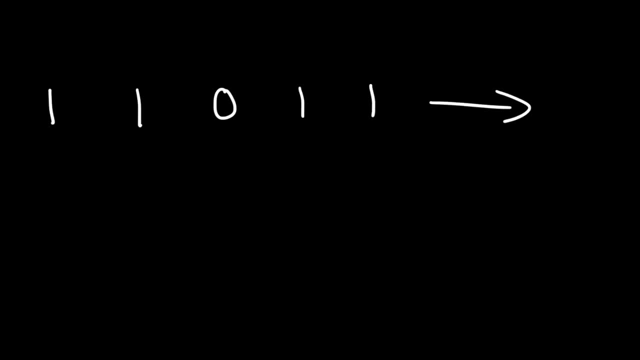 So go ahead and convert this number into a decimal number, So this is going to be 2 to the 0 times 1.. And then 2 to the 1st power times 1.. 2 squared times 0.. 2 to the 3rd times 1.. 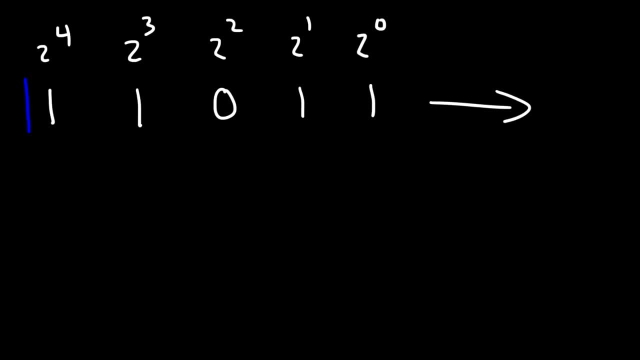 And then 2 to the 4th times 1.. And, just like before, we are going to ignore the 0 values and focus on the numbers that have a binary value of 1.. So this is going to be 2 to the 4th. 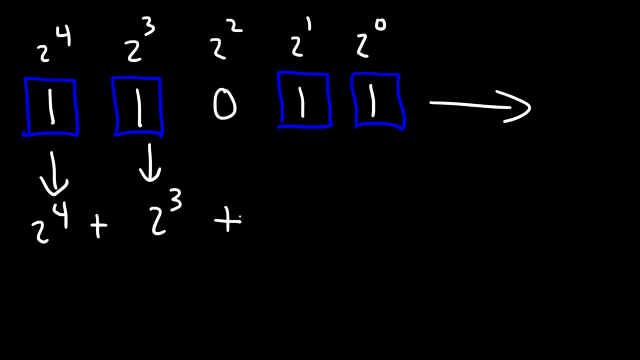 And then plus 2 to the 3rd power, And then plus 2 to the 1st, And then plus 2 to the 0 power. So, based on that table, we're going to have a binary number of 1.. 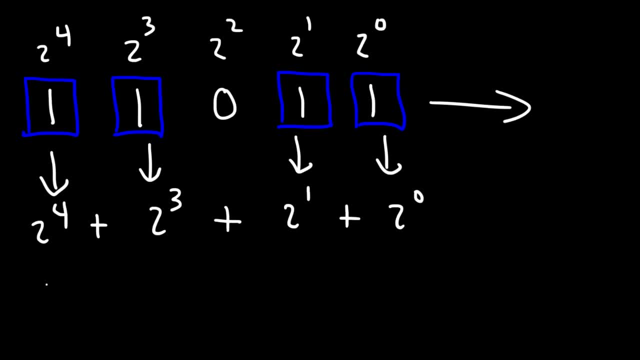 So, based on that table, or rather the information on the last page, we said that 2 to the 4th power is 16.. 2 to the 3rd is 8.. 2 to the 1st is 2.. 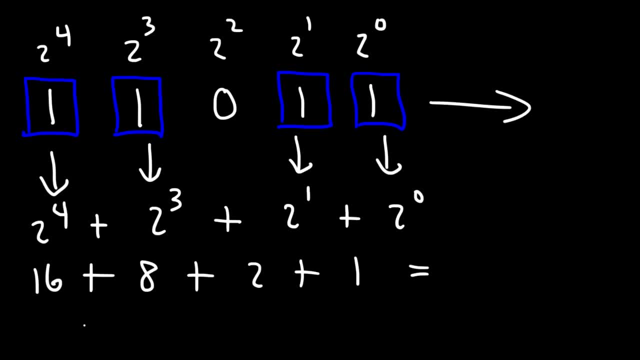 And 2 to the 0 is 1.. So now let's add: 16 plus 8 is 24.. And then 2 plus 1 is 3.. So the final answer is 27.. And so that's how we can convert a binary number into a decimal number. 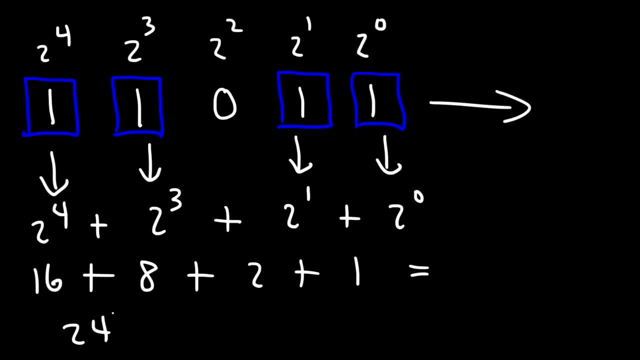 So now let's add: 16 plus 8 is 24.. And then 2 plus 1 is 3.. So the final answer is 27.. And so that's how we can convert a binary number into a decimal number. Now, for the sake of practice, go ahead and try this. 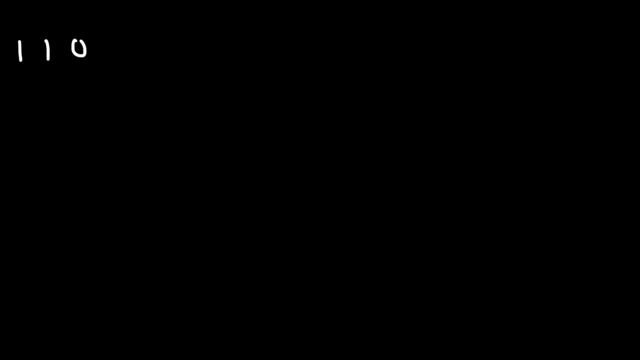 I'm going to show you how to solve these two example problems. So convert these two numbers into decimal numbers. Feel free to pause the video and work on these problems. So let's start with the first example on the left. So I like to space out the numbers. 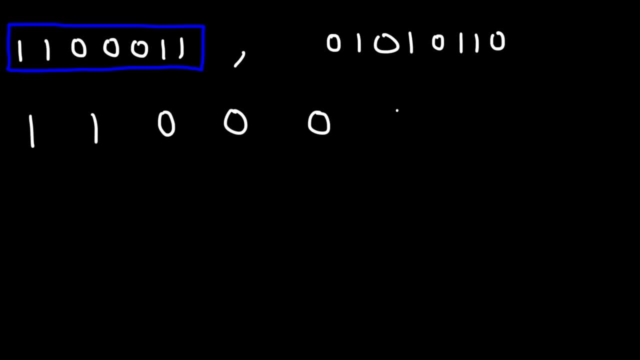 It makes it easier. So this number is going to be associated with 2 to the 0, and then 2 to the 1st, And then we're going to follow the same process for all of the other examples. And now let's focus on the numbers that contain a 1.. 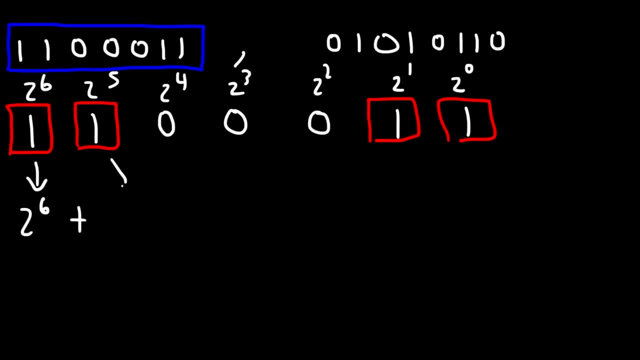 So what we have is 2 to the 6th plus 2 to the 5th power, plus 2 to the 1st power. So that's a 1.. So what we have is 2 to the 6th plus 2 to the 5th power, plus 2 to the 1st power. 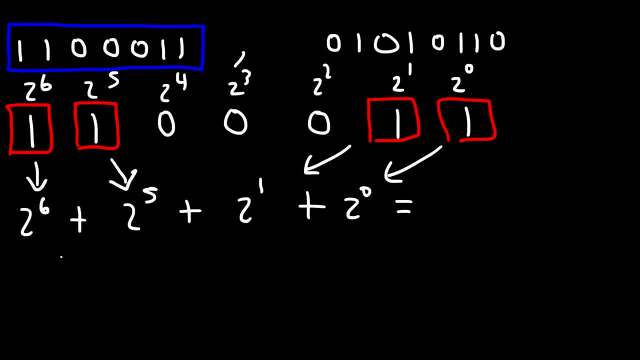 and then plus 2 to the 0 power, So 2 to the 6th power. we said that's 64.. 2 to the 5th is 32, and then plus 2 plus 1.. Now 64 plus 32,, that's 96.. 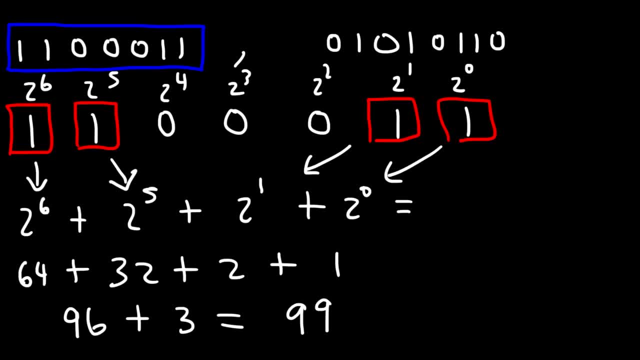 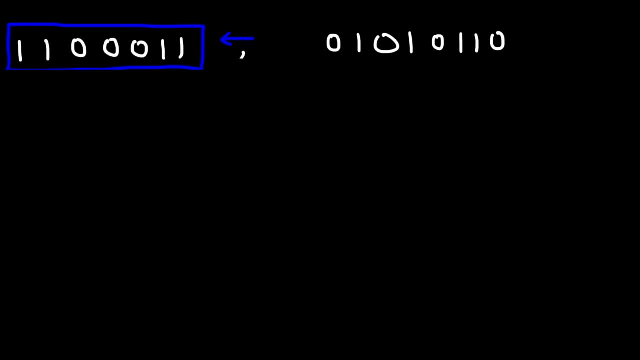 2 plus 1 is 3.. And so the final answer for the first example is 99.. And so that's it for this one. Now let's move on to the next one. So let's rewrite the number, So we have 0, 1, 0, 1, 0, 1, 1, 0. 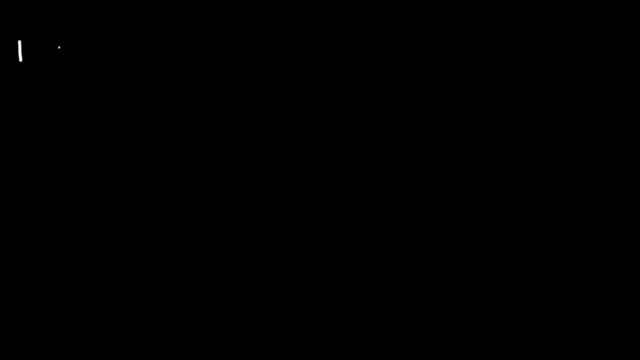 Now, for the sake of practice, we're going to use a binary number. So, for the sake of practice, go ahead and try these two example problems. So convert these two numbers into decimal numbers. Feel free to pause the video and work on these problems. 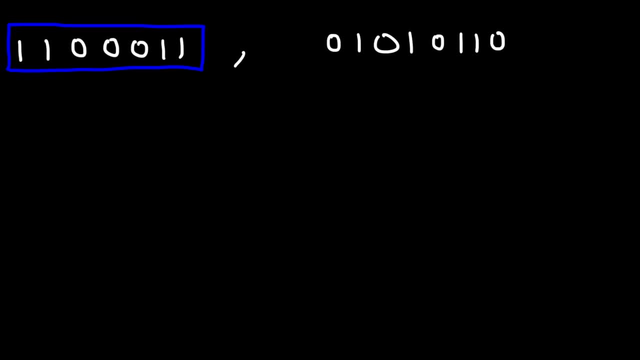 So let's start with the first example on the left. So I like to space out the numbers. It makes it easier. So this number is going to be associated with 2 to the 0 and then 2 to the 1st. 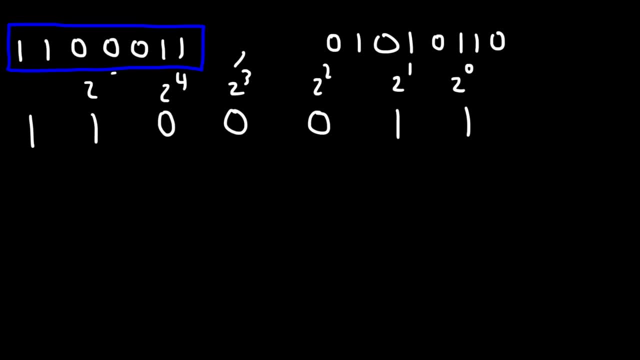 And then we're going to follow the same process for all of the other examples, And now let's focus on the numbers that contain a 1.. So what we have is 2 to the 6th plus 2 to the 5th power. 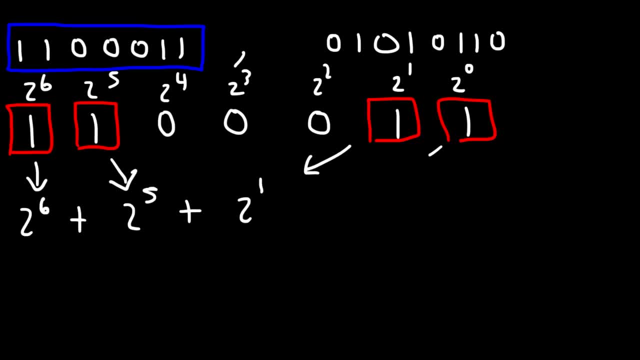 Plus 2 to the 1st power, And then plus 2 to the 0 power, So 2 to the 6th power. we said that's 64.. 2 to the 5th is 32.. And then plus 2 plus 1.. 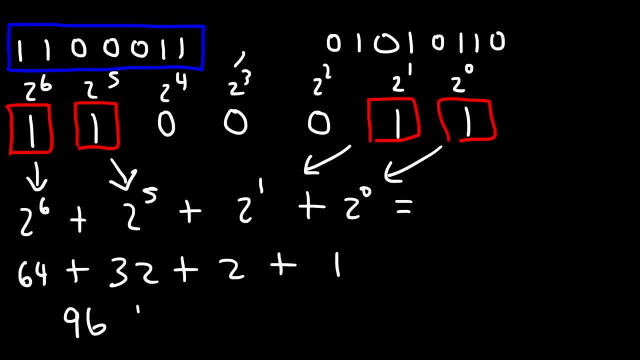 Now, 64 plus 32,, that's 96.. 2 plus 1 is 3.. And so the final answer for the first example is 99.. And so that's it for this one. Now let's move on to the next one. 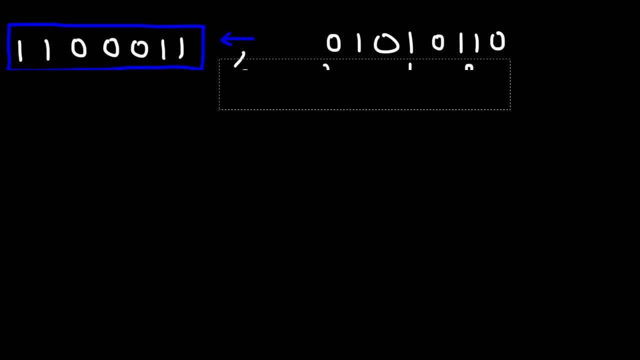 So let's rewrite the number. So we have 0, 1, 0, 1, 0, 1, 1, 0.. Now let's write these numbers at the top And once again, let's focus on the numbers that contain a 1.. 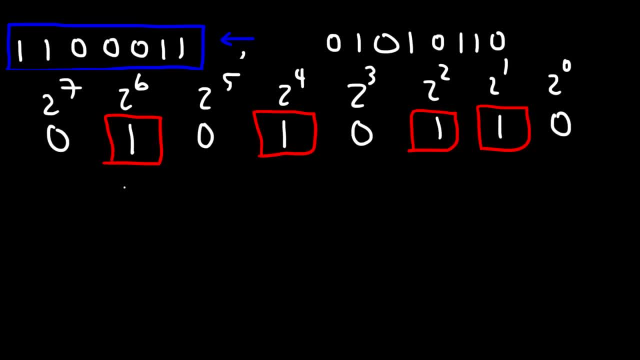 Now let's add up these numbers. So this is going to be 2 to the 6th plus 2 to the 4th power, Plus 2 squared, And then plus 2 to the 1st power. So 2 to the 6th is 64.. 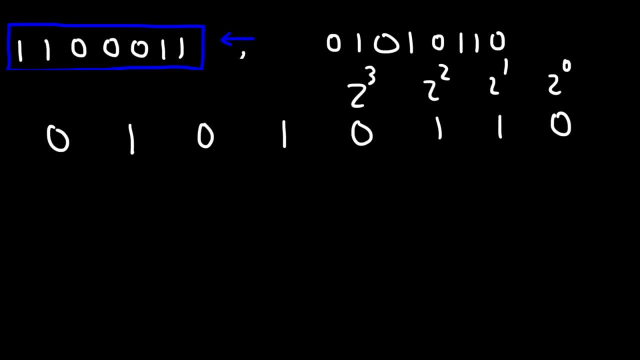 Now let's write these numbers at the top And once again let's focus on the numbers that contain a 1.. Now let's add up these numbers, So this is going to be 2 to the 6th plus 2 to the 4th power, plus 2 squared, and then plus 2 to the 1st power. 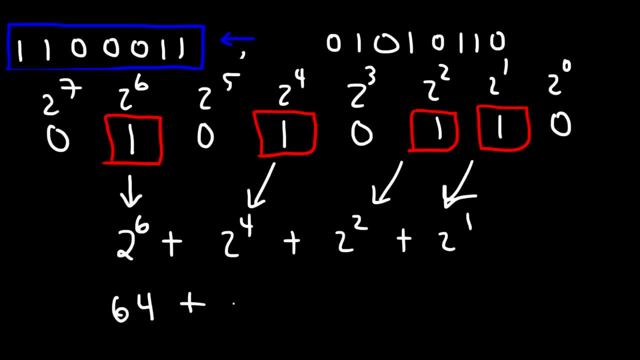 So 2 to the 6th is 64,, 2 to the 4th is 16,, 2 squared is 4, and 2 to the 1st is 2.. So 64 plus 16.. That's going to be 80.. 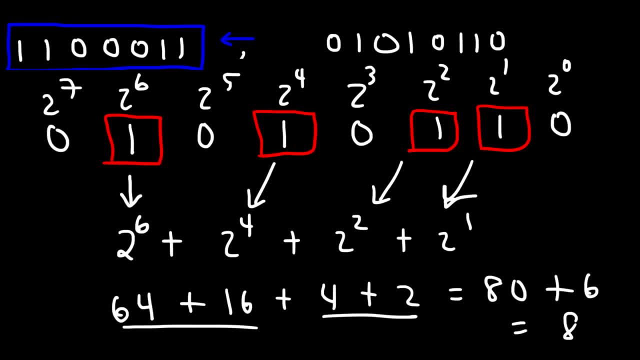 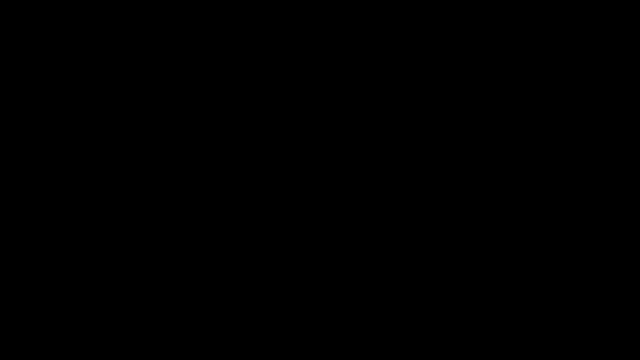 And then 4 plus 2 is 6.. So the final answer for this example is 86.. Now what if you're given a fractional binary number? How can you convert that into a decimal number? For instance, let's say we have the number 1, 1, 0, 0, with a decimal point, and then 1, 0, 1.. 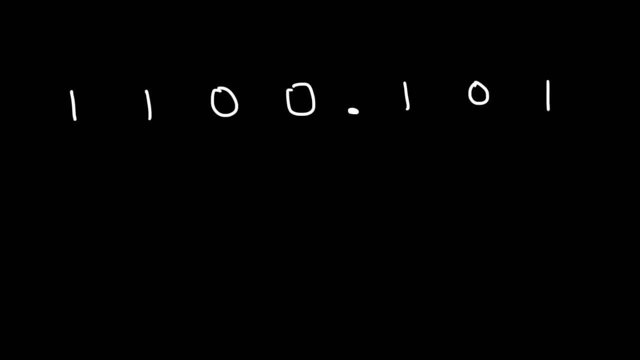 How can we convert that into a decimal number? So the first number that's to the left of the decimal point, that's 2 to the 0,, as always, And then 2 to the 1st, 2 squared, and the last one is associated with 2 to the 3rd. 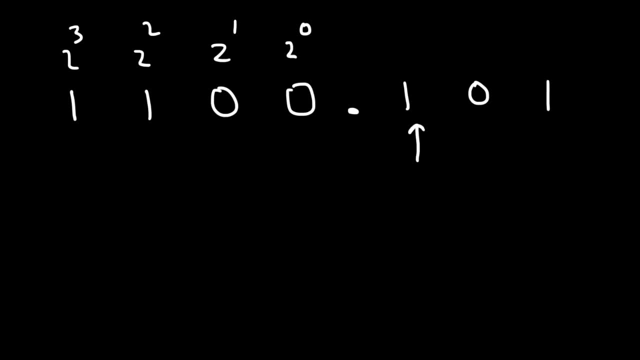 But what about the numbers to the right of the decimal? Well, if we follow the pattern of exponents that we see here, the number that's less than 0 is negative 1.. So this has to be associated with 2 to the minus 1, and then to the minus 2, and then 2 to the minus 3.. 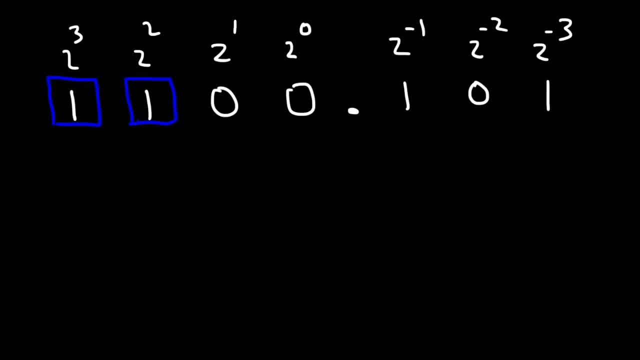 Just like before, we're going to focus on the values that bear a 1.. And so we're going to add 2 to the 3rd, plus 2 squared, plus 2 to the minus 1, plus 2 to the minus 3.. 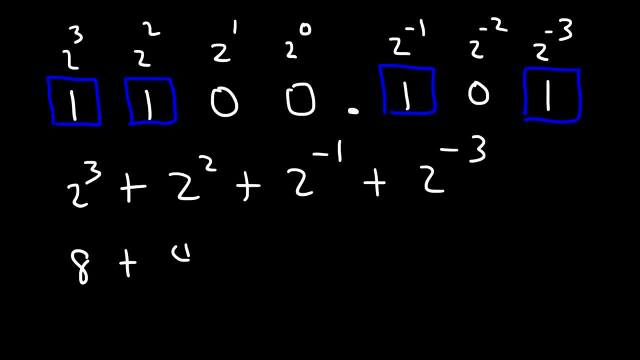 Now, 2 to the 3rd is 8, and 2 squared is 4.. But now what is 2 to the minus 1?? We know, 2 to the 1st power is 2, so 2 to the negative 1st power is 1 over 2.. 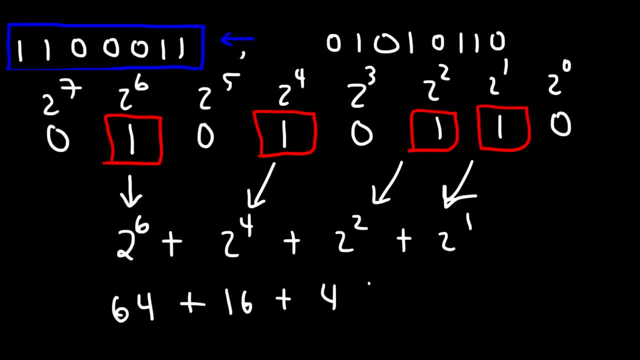 2 to the 4th is 16.. 2 squared is 4.. And 2 to the 1st is 2., So 64.. So 64 plus 16. That's going to be 80. And then 4 plus 2 is 6.. 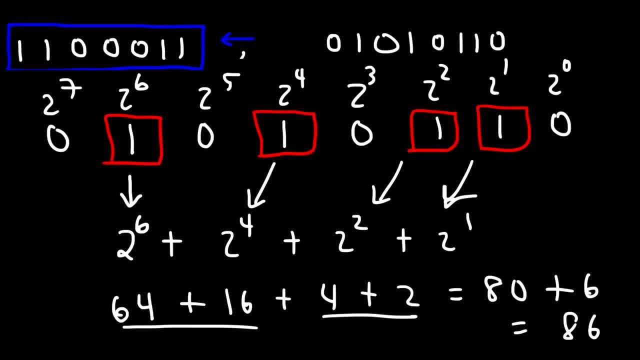 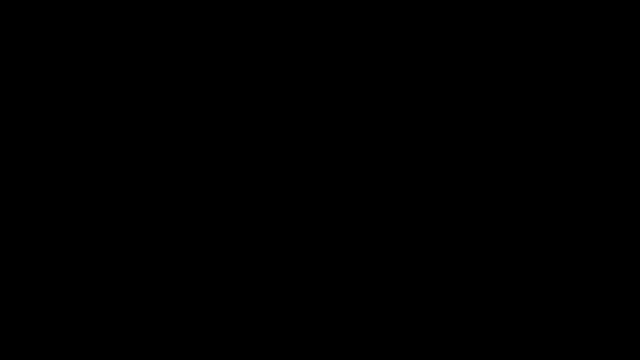 So the final answer for this example is 86.. Now, what if you're given a fractional binary number? How can you convert that into a decimal number? For instance, let's say we have the number 1, 1,, 0,, 0, with a decimal point. 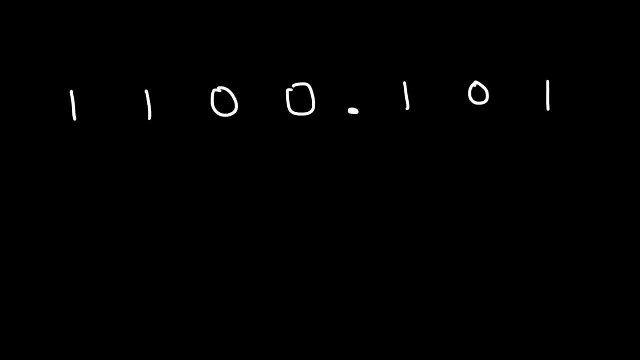 And then 1, 0, 1.. How can we convert that into a decimal number? So the first number that's to the left of the decimal point, That's 2 to the 0,, as always, And then 2 to the 1st 2 squared. 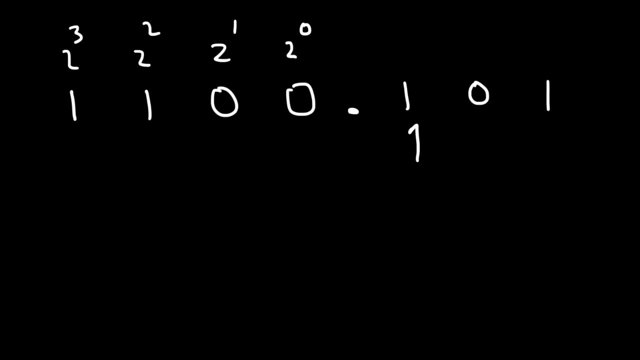 And the last one is associated with 2 to the 3rd. But what about the numbers to the right of the decimal? Well, if we follow the pattern of exponents that we see here, the number that's less than 0 is negative. 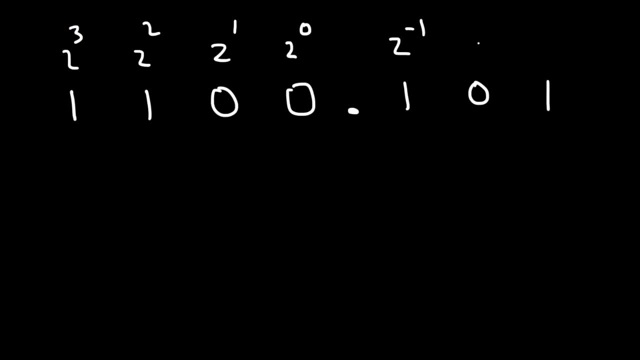 So this has to be associated with 2 to the minus 1, and then to the minus 2,, and then 2 to the minus 3.. Just like before, we're going to focus on the values that bear a 1.. 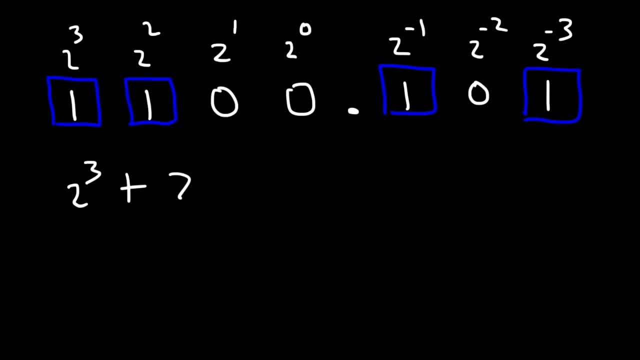 And so we're going to add 2 to the 3rd, plus 2 squared, plus 2 to the minus 1, plus 2 to the minus 3.. Now, 2 to the 3rd is 8, and 2 squared is 4.. 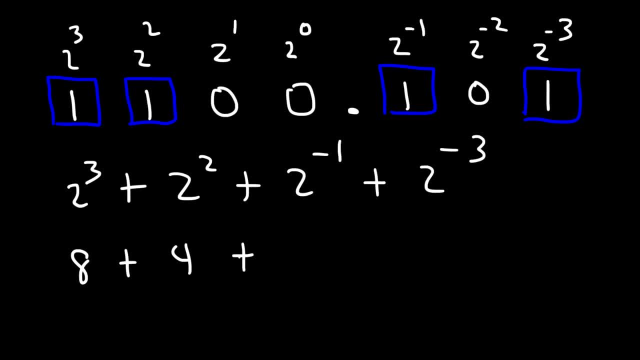 But now what is 2 to the minus 1?? We know, 2 to the 1st power is 2, so 2 to the negative 1st power is 1 over 2.. Now 2 to the 3rd is 8,. 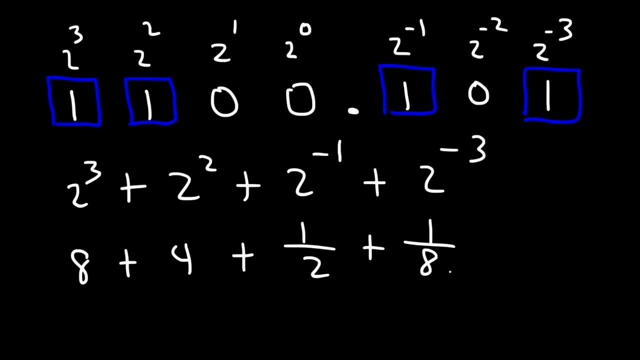 so 2 to the negative. 3rd is going to be 1 over 8.. And so 8 plus 4 is 12, and then we have 1 half plus 1 over 8.. 1 over 2, if you type that in your calculator, that's 0.5.. 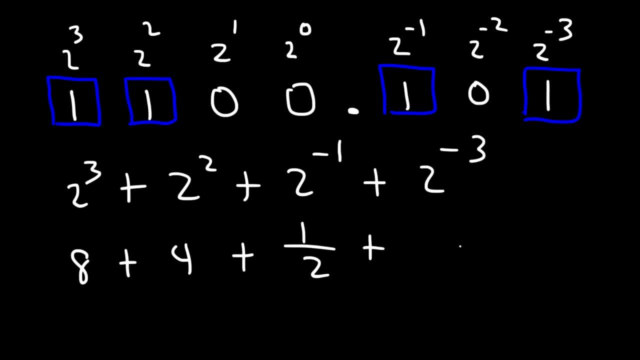 Now, 2 to the 3rd is 8,, so 2 to the negative 3rd is going to be 1 over 8.. And so 8 plus 4 is 12, and then we have 1 half plus 1 over 8.. 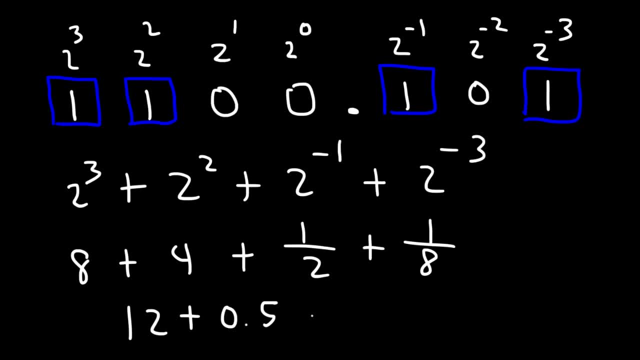 1 over 2, if you type that in your calculator, that's 0.5.. And 1 over 8, 1 divided by 8. And 1 over 8 is 0.125.. So adding up these three numbers will give us this answer. 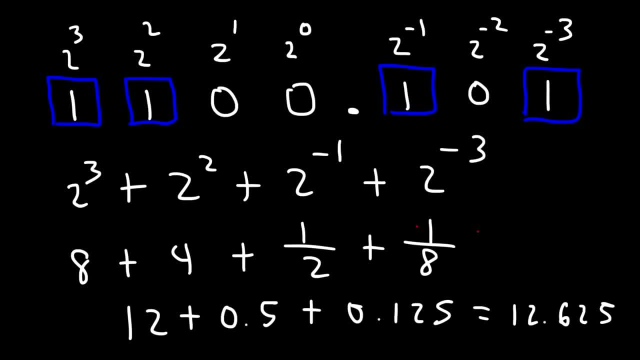 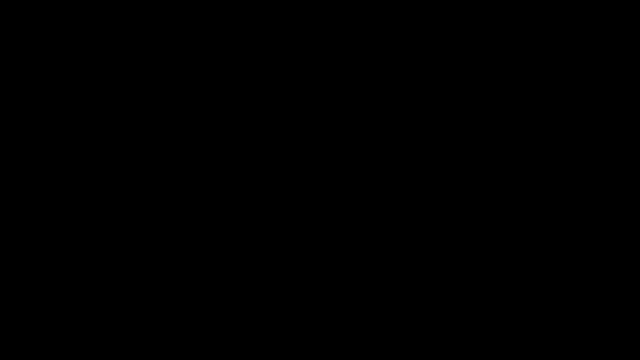 12.625.. And so that's how we can convert a fractional binary number into a decimal number Now. earlier we said that 2 to the 4th is 16.. So 2 to the negative 4 is going to be 1 over 16.. 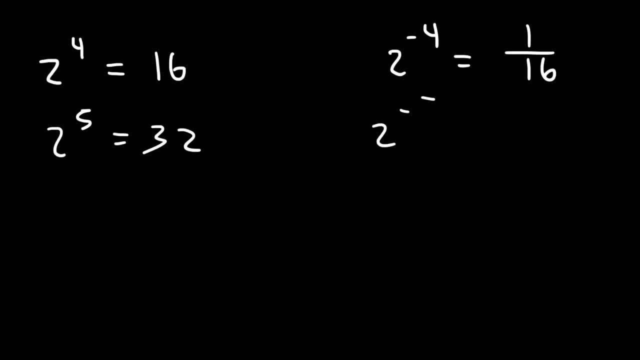 2 to the 5th is 32.. 2 to the negative 5th is 1 over 32.. So notice the pattern that you see here. 2 to the 6th is 64.. 2 to the negative 6th is 1 over 64.. 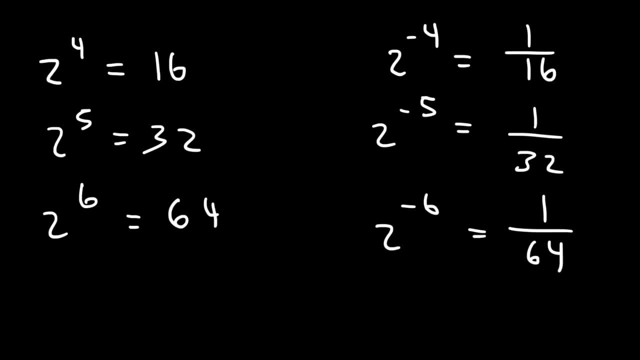 And so forth. So when dealing with fractional binary numbers, whenever you have negative exponents, just consider the ones with a positive exponent. So if 2 to the 7th is 128, then you know 2 to the negative 7th is just 1 over 128.. 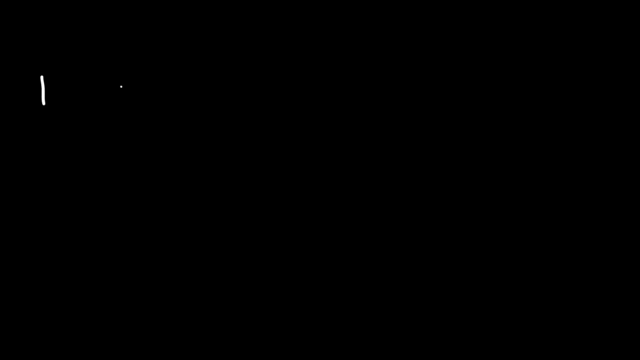 So here's another example that you could try: 1, 0, 0, 1, 1, 0, 1, 1.. Go ahead and convert that into a decimal number. So let's begin by putting the appropriate values next to each number. 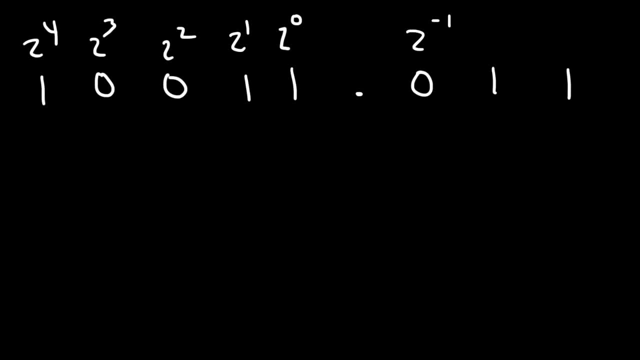 So on the left it's going to be 2 to the minus 1.. 2 to the minus 2. And 2 to the minus 1. And 2 to the minus 3.. So let's focus on only the ones that we see. 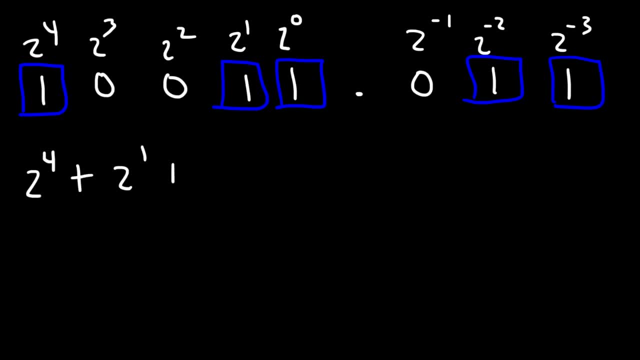 So it's going to be 2 to the 4th power, plus 2 to the 1st power, plus 2 to the 0 power, And then plus 2 to the minus 2, plus 2 to the minus 3.. 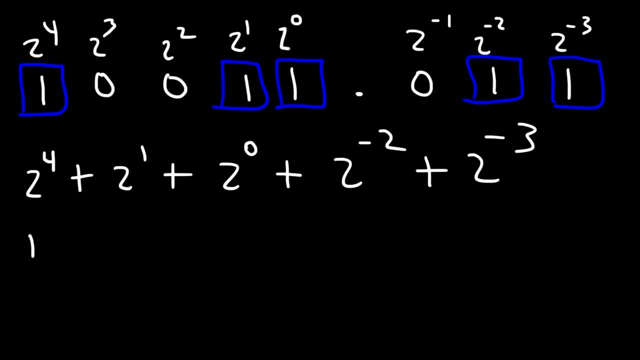 2 to the 14, I mean not 14,, but 2 to the 4th- power is 16.. And 2 to the 1st power is 2.. 2 to the 0, power is 1.. And then 2 to the negative 2.. 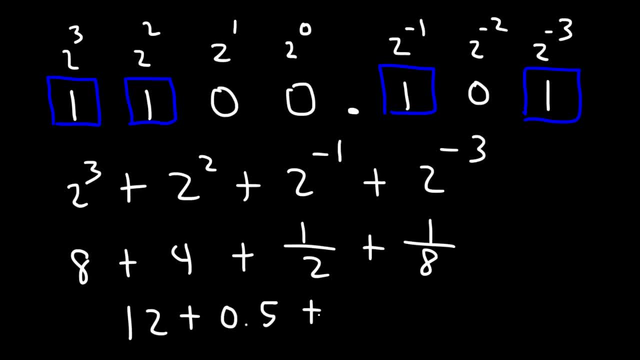 And 1 over 8,, 1 divided by 8, is 0.125.. So adding up these three numbers will give us this answer: 12.625.. And so that's how we can convert a fractional binary number into a decimal number. 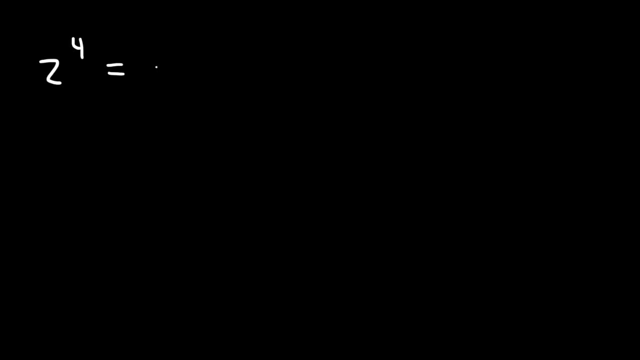 Now, earlier we said that 2 to the 4th is 16.. So 2 to the negative 4 is going to be 1 over 16.. 2 to the 5th is 32.. 2 to the negative 5 is 1 over 32.. 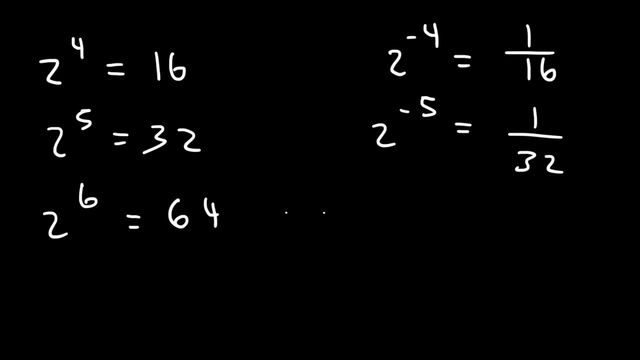 So notice the pattern that you see here: 2 to the 6th is 64.. 2 to the negative 6th is 1 over 64. And so forth. So when dealing with fractional binary numbers, whenever you have negative exponents, 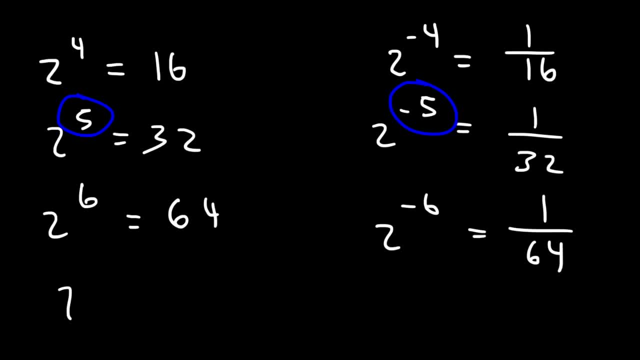 just consider the ones with a positive exponent. So if 2 to the 7th is 128, then you know 2 to the negative 7th is just 1 over 128.. So here's another example that you could try. 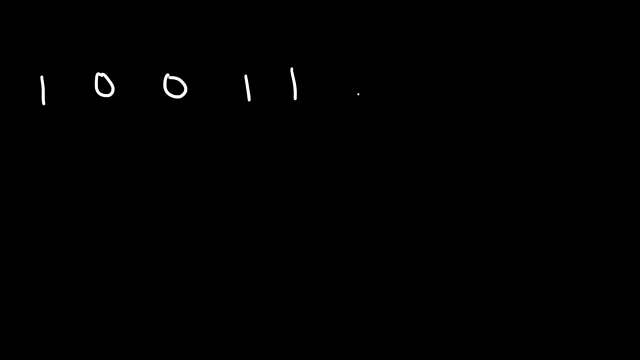 1, 0, 0, 11 point 0, 11.. Go ahead and convert that into a decimal number. So let's begin by putting the appropriate values next to each number. So on the left it's going to be 2 to the minus 1.. 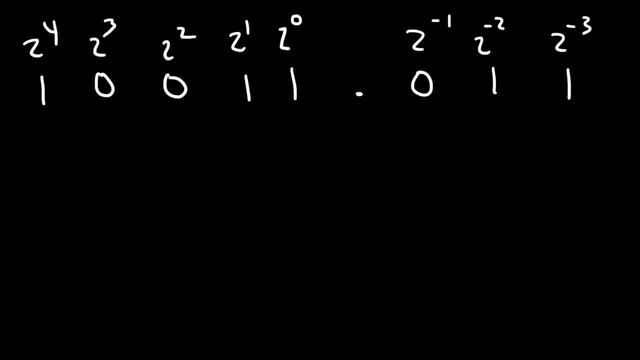 2 to the minus 2. And 2 to the minus 8.. 2 to the minus 9.. to the minus 3.. So let's focus on only the ones that we see. So it's going to be 2 to 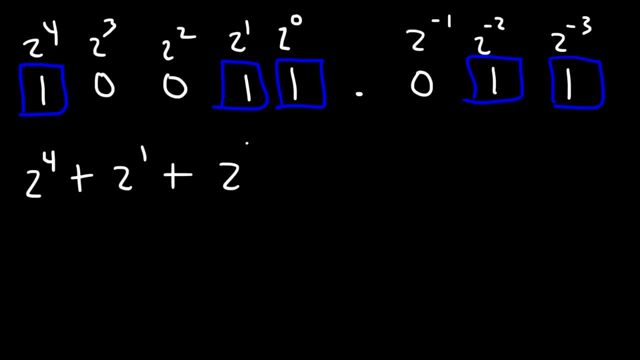 the 4th power, plus 2 to the 1st power, plus 2 to the 0 power, and then plus 2 to the minus 2, plus 2 to the minus 3.. 2 to the 14, I mean not 14,, but 2 to the 4th power is 16 and 2. 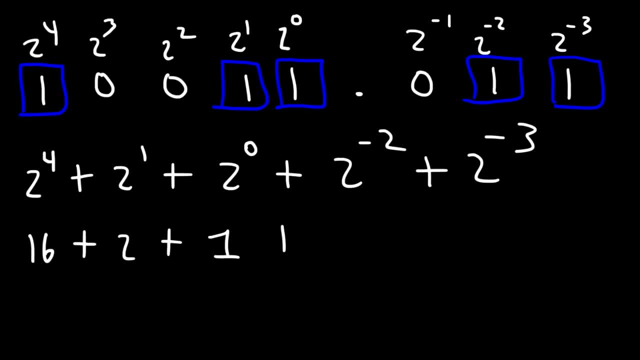 to the 1st power is 2.. 2 to the 0 power is 1, and then 2 to the negative, 2.. If 2 squared is 4,, 2 to the negative, 2 is 1 over 4.. And if 2 to the 3rd power is 8,, 2 to the negative.